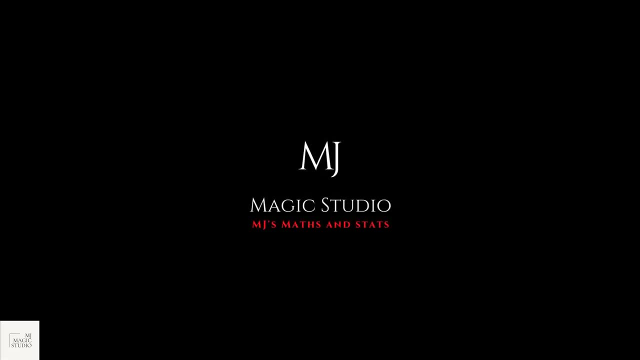 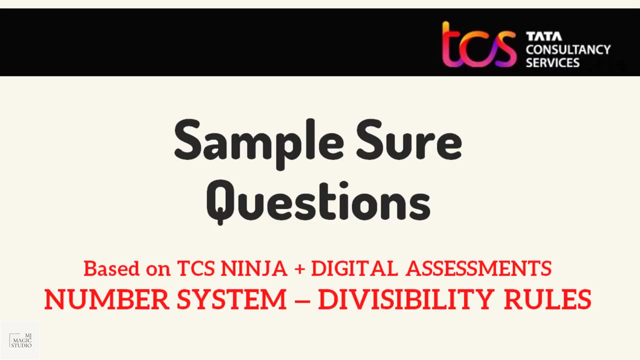 Hello everyone and welcome once again to MJ's Maths and Stats, That's MJ Magic Studio. to you, I am your host, your dost and, as usual, in the ghost mode, Mohit Jain. Today we would be discussing few questions and the formats of these questions which are regularly asked on TCS level examination. 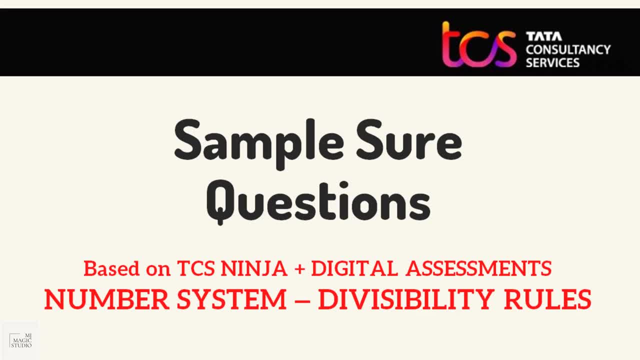 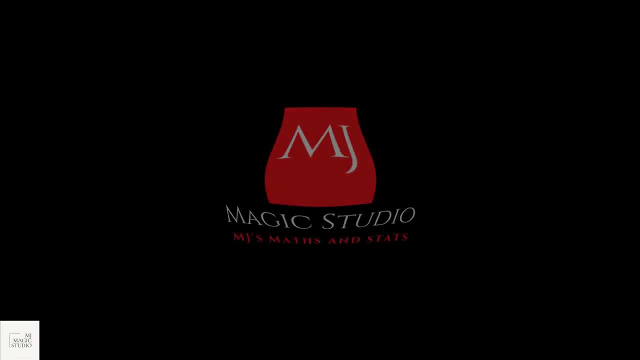 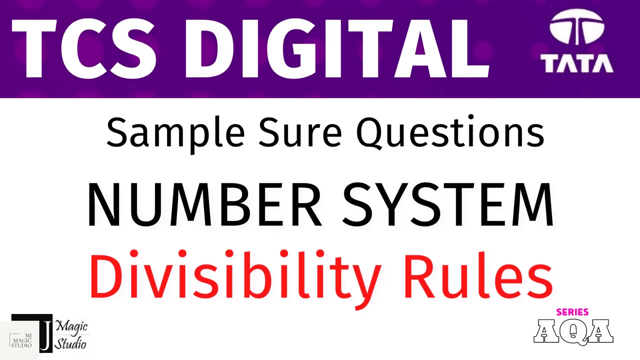 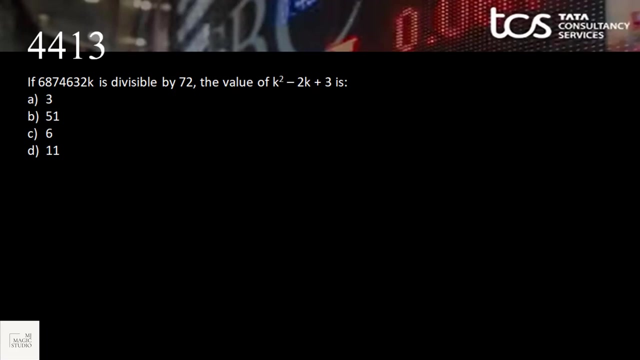 be it NQT or off-campus or BPS, Smart Hiring on TCS ION platform or you can also get these type of questions in any examination. So, on the high demand, we have taken up this number system and this session will be on divisibility. 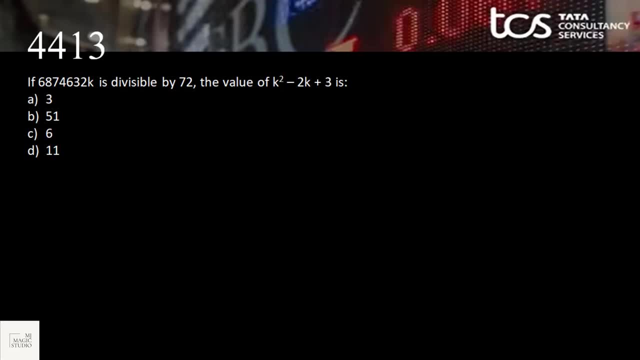 rules and you know the drill. Please look at the question, try to solve it yourself, and then we will see the solution. If a number is given is divisible by 72,, a number is said to be divisible by 72 when it is divisible by 8 and it is also divisible by 9.. 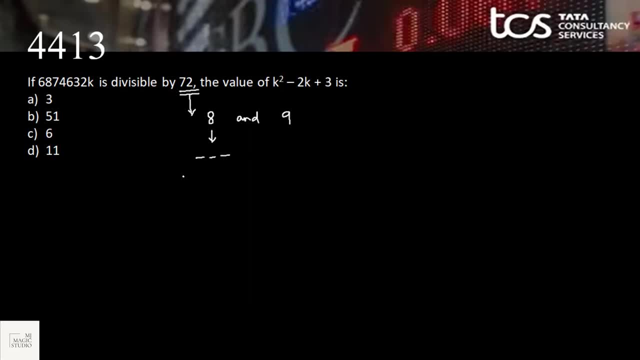 Rule for 8 is last 3 digits should be divisible by 8. That means 3,, 2, k should be divisible by 8.. We can have 320 which is divisible by 8, and we also have 328 which is divisible. 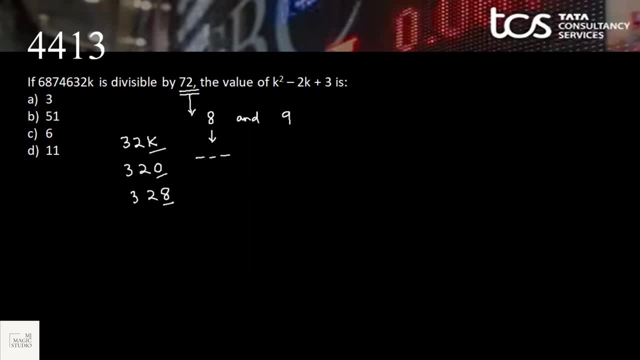 by 8.. So for now we have got 2 values of k. Now we also need to check that this number should be divisible by 9, and rule for divisible by 9 is sum of digits should be divisible by 9.. So we have 6,, 8,, 7,, 4,, 6,, 3,, 2, k. Make pair of 9 and eliminate 9 gone, 9 gone, 8 plus. 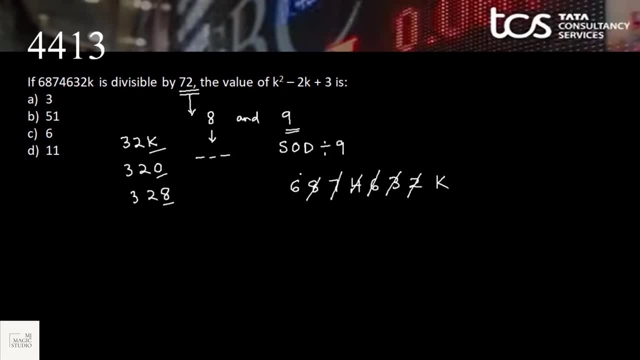 4 is 12, and 1 plus 2 is 3,. 3 plus 6 is 9.. That means this total is divisible by 9.. Value of k is 0.. We can't take value of k as 8,. we can't take value of k as 9, we can't take. 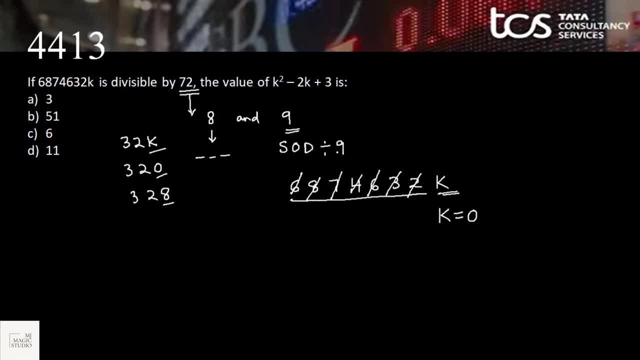 value of k as 8.. If we take k as 8, this number won't be divisible by 9.. If k is 0,, this number is divisible by 9.. That means value of k is 0.. Now the question is what? 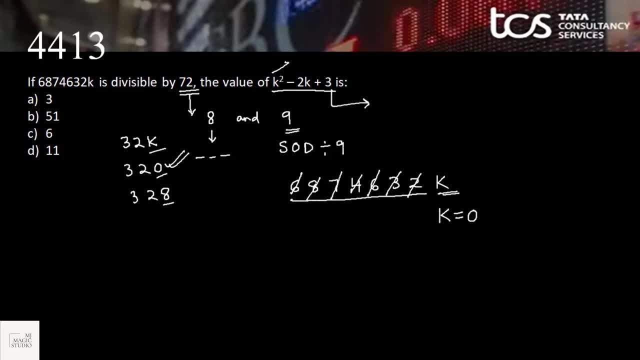 is the value of k square minus 2k plus 3?? Obviously, value of k is 0.. Then the value of the entire quadratic expression is 3.. We go with option a. Ok, what we have now? what is the value of 5x plus 9y if four-digit number x, 4,, 7, y? 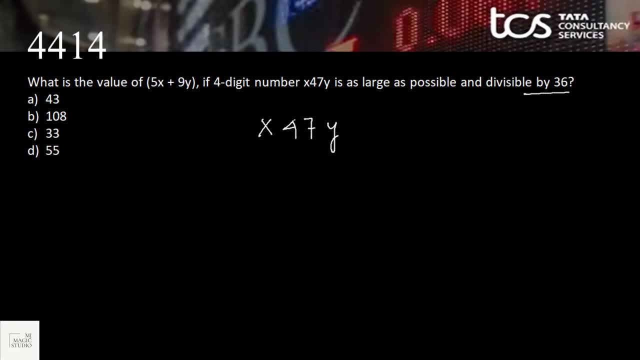 is as large as possible and divisible by 36?. First of all, a number is divisible by 36 only when it is divisible by 4 and 9.. A number is divisible by 4 when last two digits are divisible by 4.. 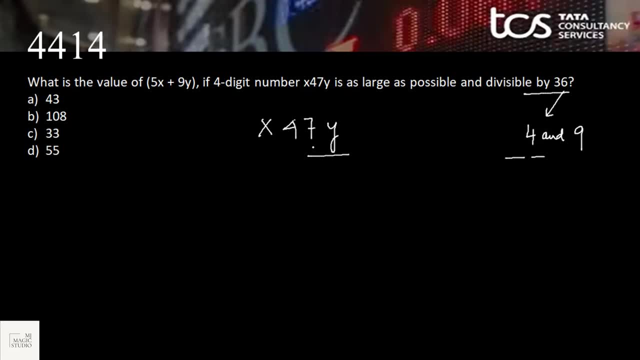 That means 7y1. is divisible by 4.. 72 is divisible by 4.. 76 is divisible by 4.. So the highest value of y would be 6.. So if we take 6 now, we know the rule for 9.. Rule for 9 is: 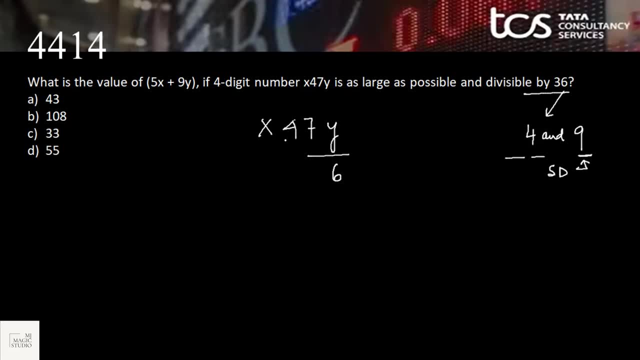 sum of digits should be divisible by 9.. So now, 6 plus 4 is 10 plus 7 is 17.. What should be the value of x so that this total becomes divisible by 9?? See 17 plus 10.. 17 plus 10 is 27, but x cannot be 10.. So 17 plus 1 will be 18.. So the largest 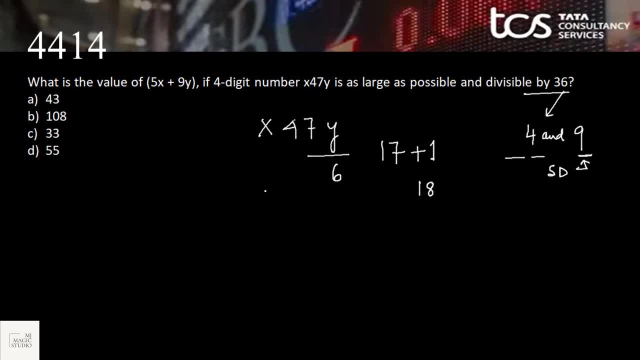 possible number which we have here is 1476.. But stop, If I take y equals to 2,, if I take y equals to 2, this become 9 plus 4, that is 13, and the value of x can be 5.. So that can be 5, 4,. 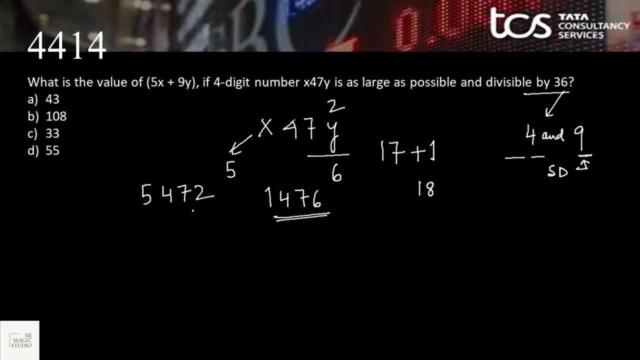 7, 2, which is divisible by 4 and which is also divisible by 9.. That means this is the highest number which we are looking out for. Value of x is 5.. This becomes 25 and value of y is 2.. 9 into 2 becomes 18.. 25 plus 18 is 43. So our 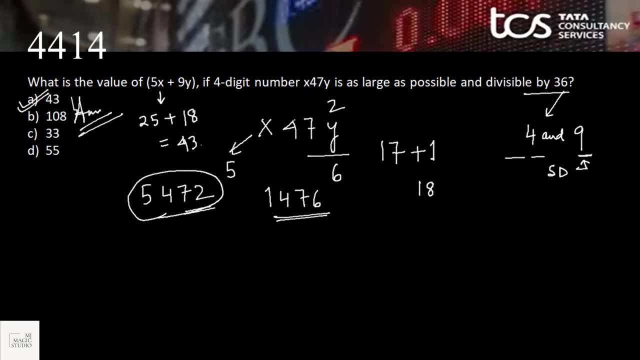 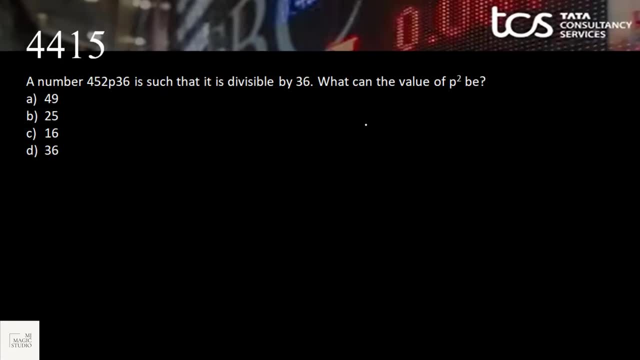 answer is 43, option A. Okay, so the next one is also here. we are looking out for the number which is divisible by 36, and we know the drill for 36.. It need to be divisible by 4 and 9, both 4, last two digits, 36,. bingo, it is divisible by 4.. We just need to make 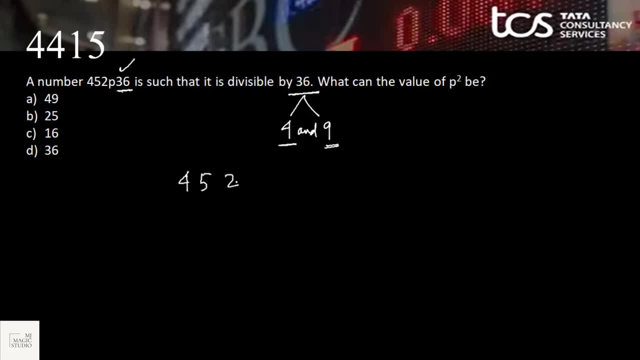 it divisible by 9.. So 4,, 5,, 2, p, 3,, 6,, 9 gone, 9 gone, 2 plus p should be equals to 9, that means value of p is 7.. If value of p is 7, then that number would be divisible. 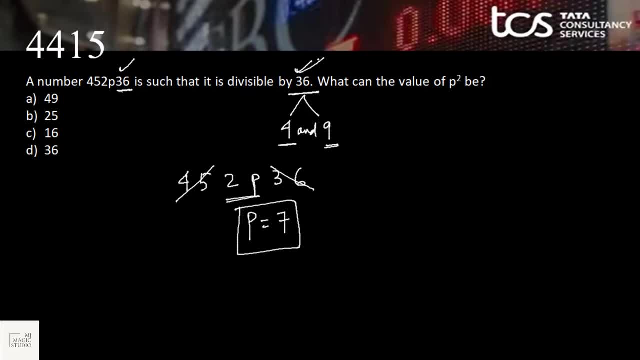 by 9 and it is divisible by 4 itself. that means it is divisible by 36.. So value of p is 7, value of p square isn't there in the question. p square is 49, option A fits it. 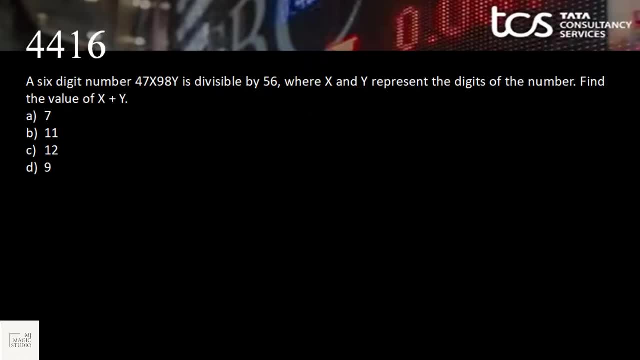 Same. Okay, I guess you are pausing the session and trying to solve by yourself. Here we have a 6 digit number and it is divisible by 56, which is again a composite number. that means the number is said to be divisible by 56 when it is divisible by 7 and 8.. We know the drill. 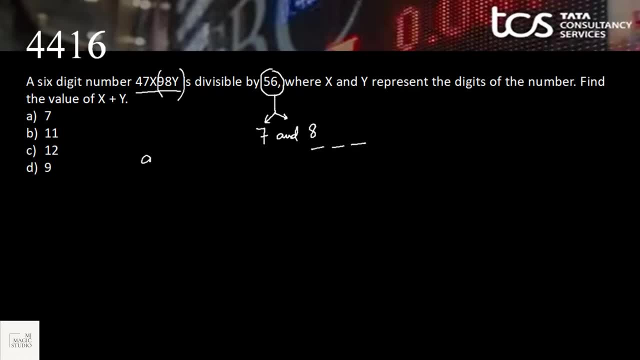 for 8,. first let us check for 8.. 9,, 8, y should be divisible by 8.. 8,, 8, y, 8,, 8,, 9,, 9,, 8, should be divisible by 8.. 8,, 18,, 16,. 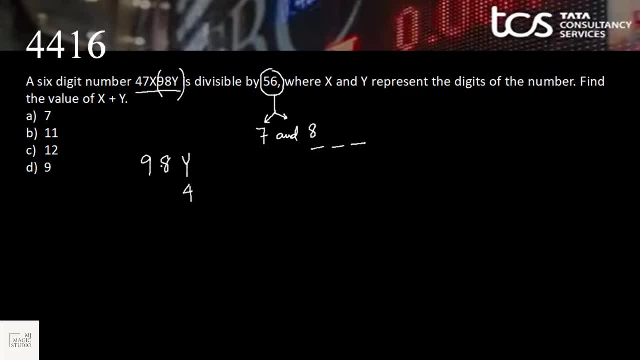 2,. that means value of y is 4.. 8,, 16,, 24.. Correct, So our number is now 4, 7, x, 9, 8,, 4.. This number is divisible by 8.. 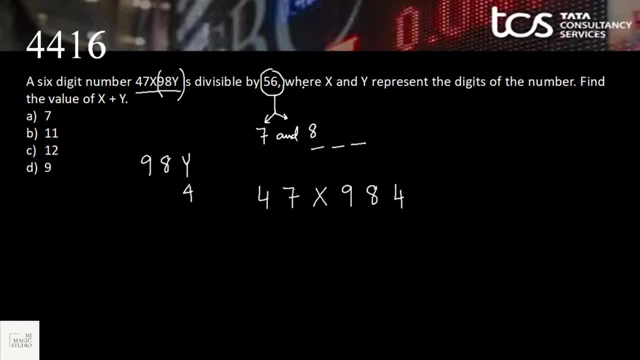 Now we need to make this number divisible by 7. And it is given that x and y represent the digits. Find the value of x plus y. Now rule for 7 is very simple: From the right hand, from sorry, left hand side, write. 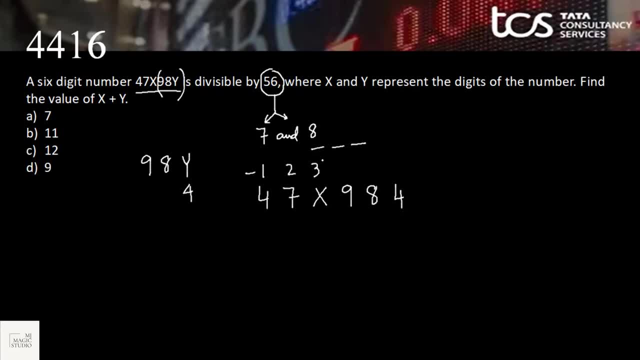 minus 1,, 2, 3 and again change the sign 1, minus 2, minus 3 as the coefficients. Now we will multiply this Minus 4 plus 14, plus 3x plus 9, minus 16, minus 12.. 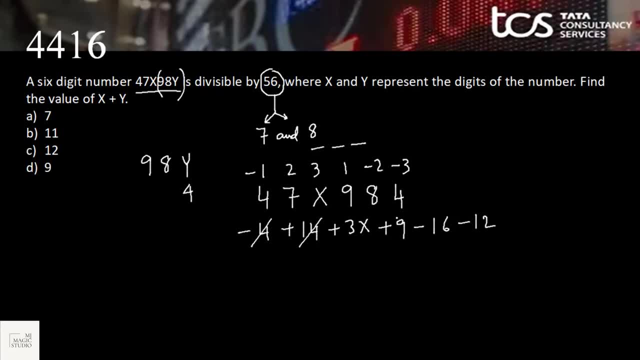 So 14,, 4, 10, and 19, 3, 15. We have got 3x minus 15.. This should be equals to 0.. If this is equals to 0, value of x is 5.. 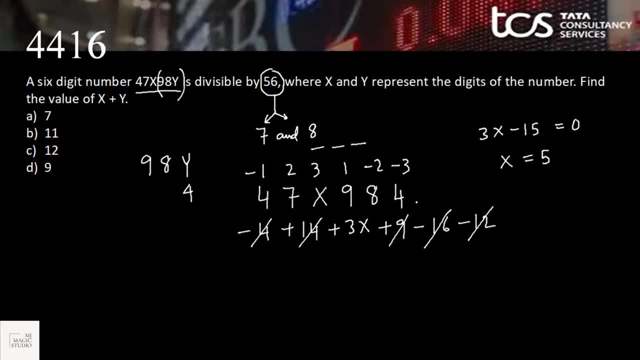 So when value of x is 5, this entire number is divisible by 7.. This is the code we use from left to right on the digits with alternative sign. We multiply these, Then we add up. The addition should be equals to 0 or multiple of 7.. 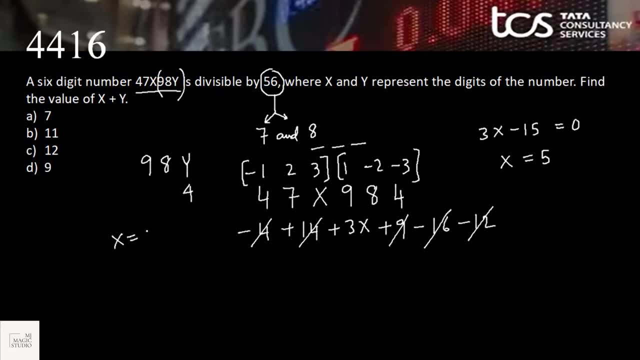 If it is 0, value of x is 5.. That means x is equals to 5.. 5 and y is equals to 4.. So x plus y is equals to 9.. We are asking for what is the value of x plus y? x plus y is equals to 9,. that is in option D. Now what we? 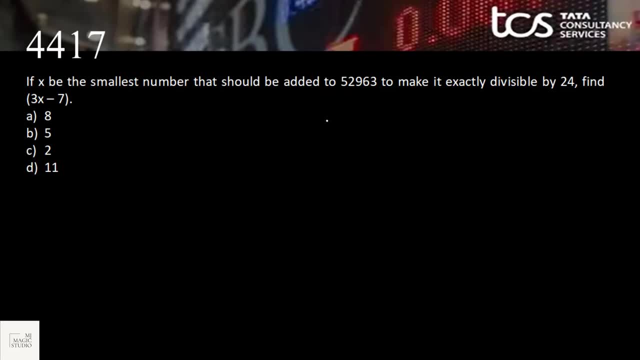 have. x is the smallest number, that should be added with 52963 to make it exactly divisible by 24.. 24 is again composite. Rule here is it should be divisible by both 3 and 8.. For 3, sum of digits should be divisible by 3 and for 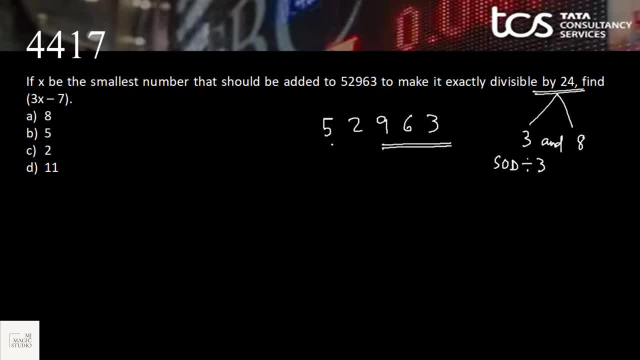 8, last 3 digits should be divisible by 8.. Now sum of digits is 7,, 10,, 19 and 625.. And 960, we know 960 is divisible by 8.. So if we add 5 to it, if we add 5 to it, it will become 52968, and this 968 is divisible by 8.. And since 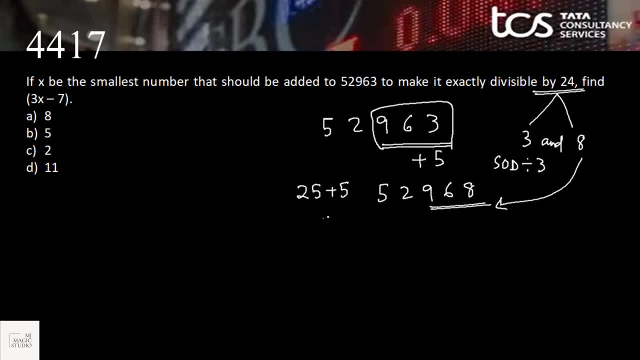 we are adding 5, sum of digits. sum of digits becomes 30,, which also give us the clue that this number is divisible by 3.. That means the smallest number we need to add is 5.. Value of x is 5.. Now find the value of 3x minus 7.. 15 minus 7 is: 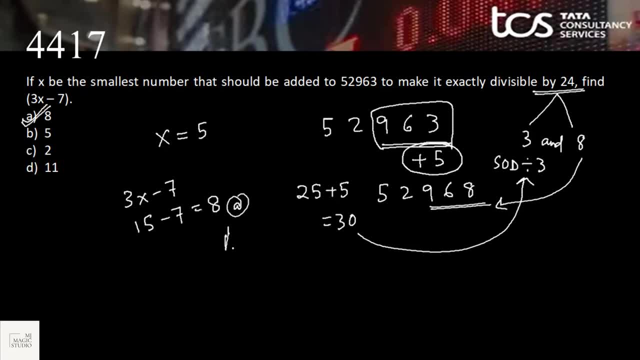 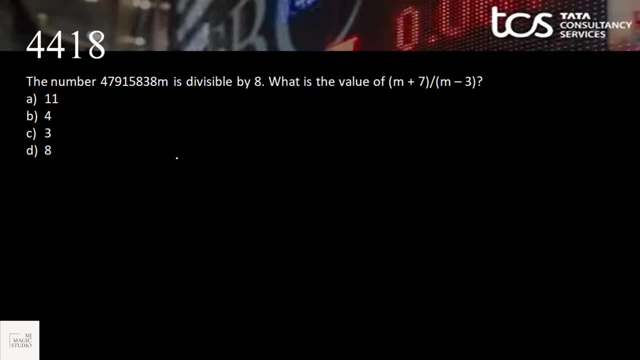 equals to 8.. Option A is the pick. Next example: The number 47915838m is divisible by 8.. Only 8 is there. That means last 3 decits should be divisible by 8.. 38m should be divisible by 8, 8 into 4.. 32 and then 2.. 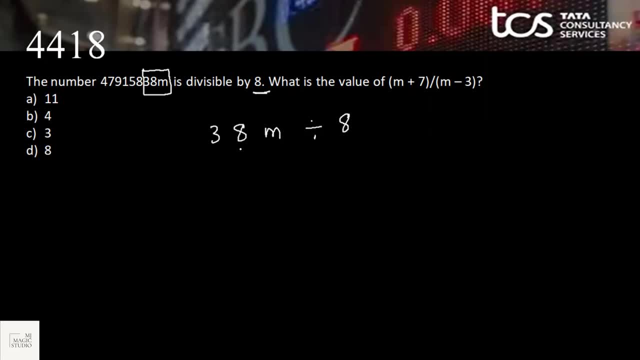 So F means 0 and 4 will be divisible by 8. And long term itself, F means 8.. So this is small, but it serves as the reason to any formula variance In fulfillment. feed up theそして p for key. Go and make a pximum or find out the p. Now see, there is 2 numbers possibilities. 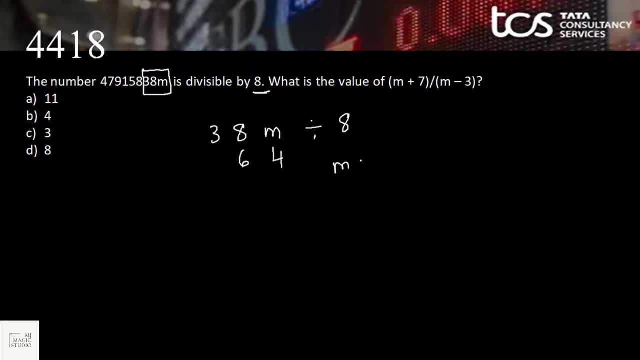 R and a P is also written, So everything here will be correct. For just multipleoodies optionừngijateed up, we will get 6,, 64. Value of m will be 4.. If value of m is 4,. 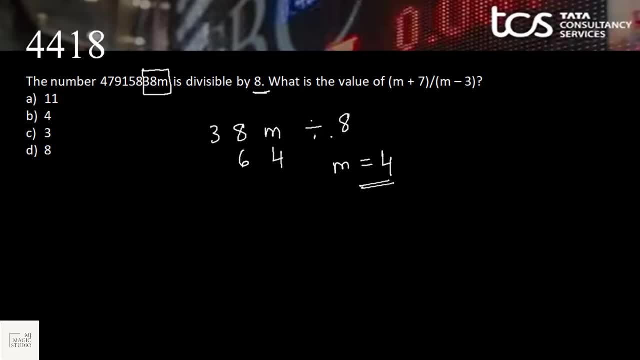 384, 3264 is divisible by 8.. That means what is the value of m plus 7 upon m minus 3? 4 plus 7 upon 4 minus 3,, that is 11 by 1.. Answer is 11,. 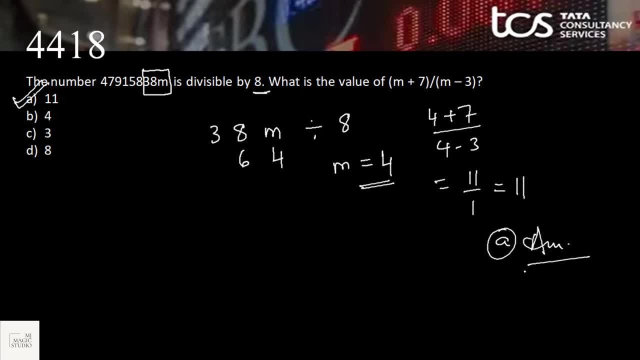 that is, in option A. A 6-digit number is exactly divisible by 7,, 11 and 13.. Wow, And the property goes like a 6-digit number, where all the digits are same, is divisible by 7,, 11 and 13. 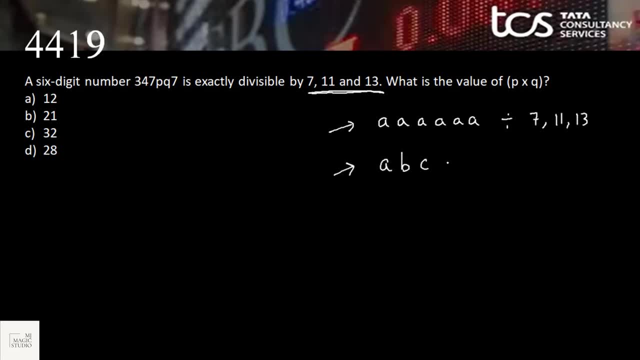 and a 6-digit number of the form ABC. ABC is divisible by 7,, 11 and 13.. If we look carefully, this is of the forms ABC. ABC. That means 3, 4, 7.. It should be 3, 4, 7.. Then this 6-digit number. 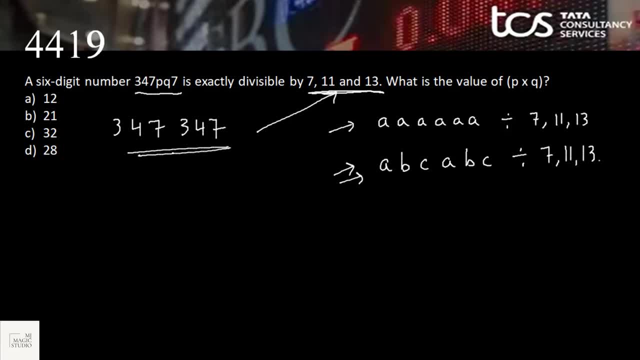 would be exactly divisible by all 3,, 7,, 11 and 13.. That means value of p is 3 and value of q is 4.. What is the value of p into q? p into q is 3 into 4,. 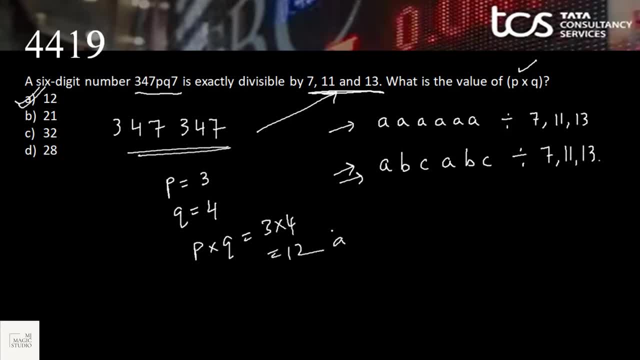 that is 12.. Option A fits again Now. we have taken example for 88. A 10-digit number is divisible by 88. That means it is divisible by both 8 and 11. We know the drill for 8.. Last 3 digits should be divisible by 8.. 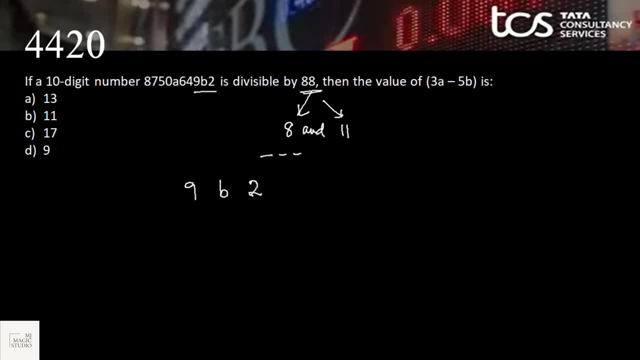 9b2.. 9,, 8 and then 32.. We have got. we need 3,, 16,, 19.. 9,, 9,, 2.. 9, 1, 2 also, I guess. 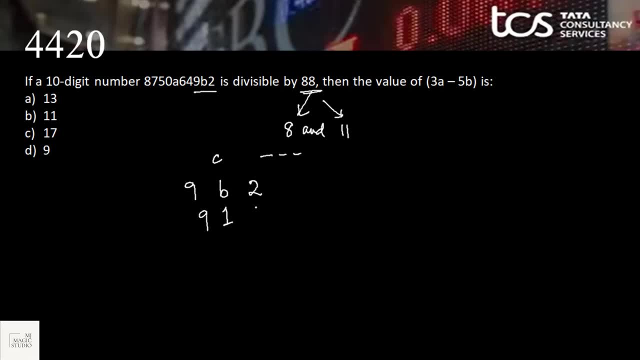 9,, 11,. yes, Value of b can be 1.. 9,, 1,, 2., 8,, 11,, 8,, 32.. Or 9,, 9,, 2., 8,, 16,, 32.. So value of b can be 1.. 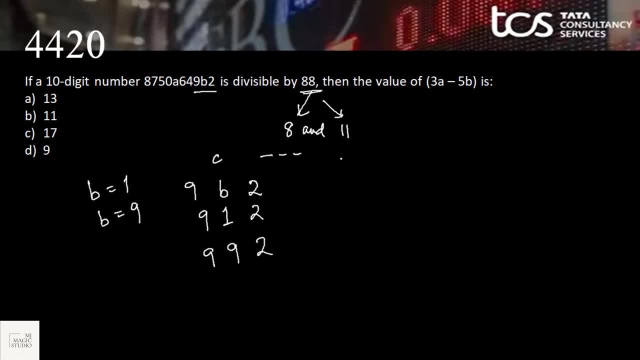 Value of b can be 9.. 9,, 9,, 2.. 8,, 16,, 32.. So value of b can be 1.. Value of b can be 9.. Now 8,, 7,, 5,, 0, a. 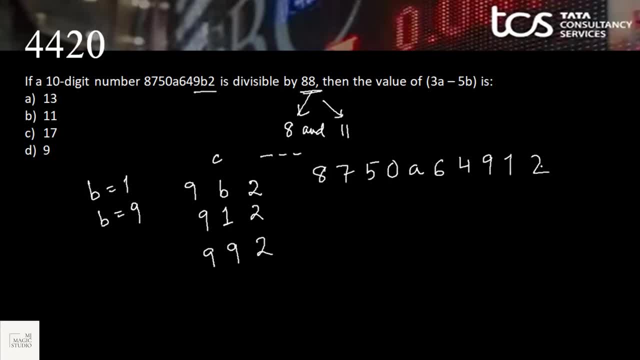 6,, 4,, 9,, 1,, 2 is divisible by 11.. And for checking the divisibility rule of 11, we know that odd placed digits minus even placed digits should be equals to 0 or divisible by 11.. 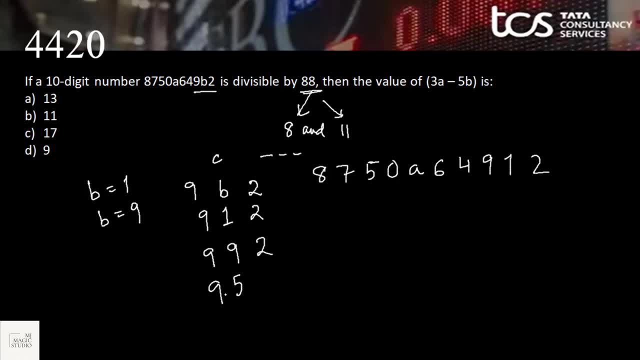 One more thing: 9, 5,, 2.. 9, 15 and then 72.. 9, 5, 2 is also divisible by 8. So value of b can be 1,, 5 or 9.. 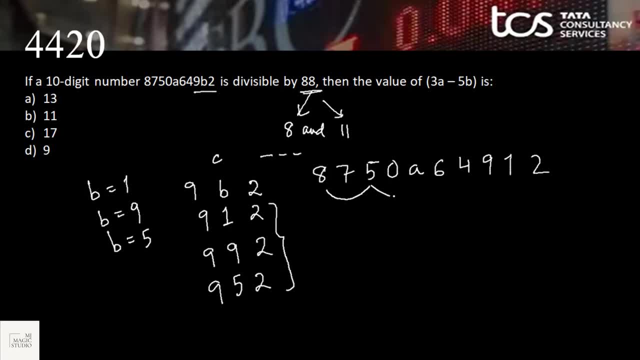 Now let us check this: 13 plus a, 17 and plus b. So this is 17 plus a plus b, And here we have 7 plus 6,, 13. And 9, 2.. 22 plus 2 is 24.. 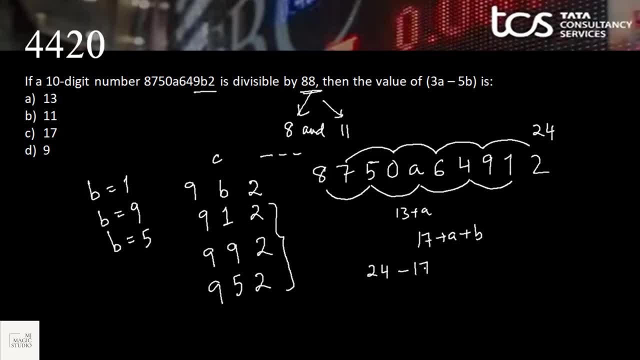 Let us find the difference: 24 minus 17 minus a minus b is equals to 7 minus a minus b. If I put this at equals to 0, then a plus b is equals to 7.. Okay, So b is 1.. 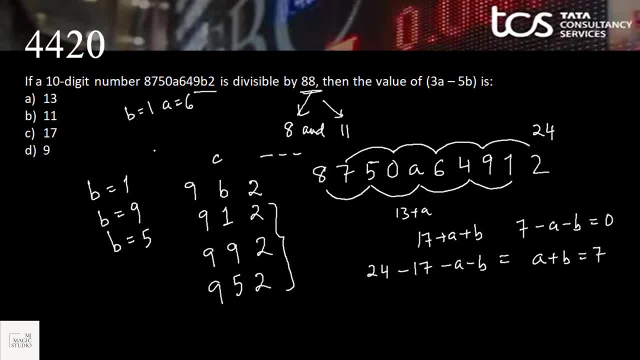 a can be equals to 6.. So 18 minus 5 can be equals to 13.. Which is there in the option? If I take b, equals to 5, a can be equals to 2.. 6 minus 25, it is coming as negative. 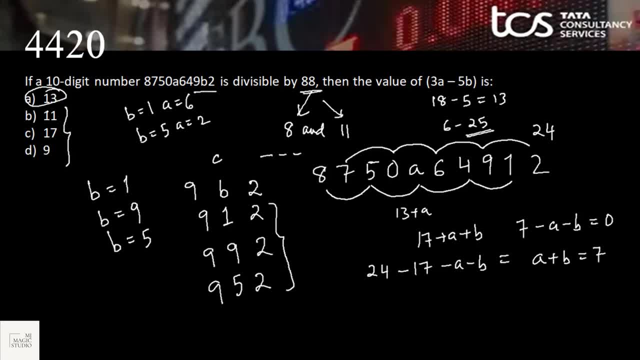 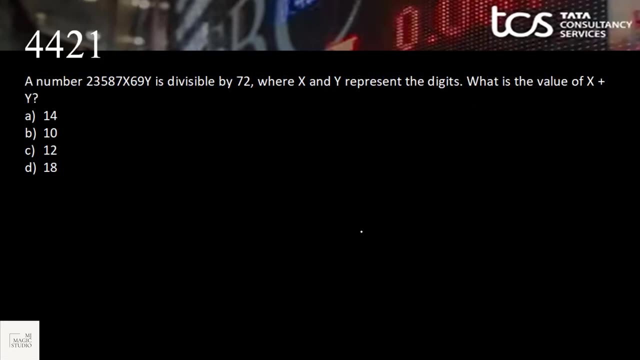 Then there are no negatives, Since we have got one of the option which is there. we take it as b equals to 1 and a equals to 6.. And the answer is 13.. Okay, One more example For 72, and we know the drill for 72.. 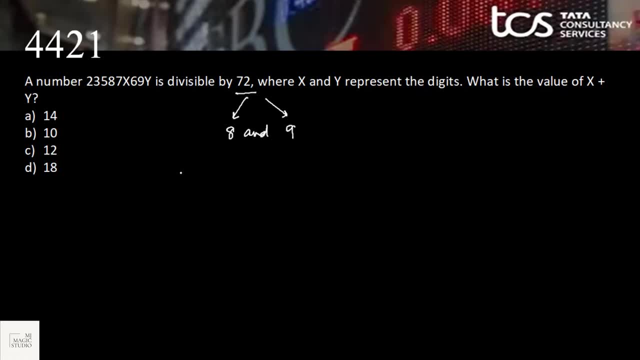 Number should be divisible by 8 and 9.. So first let us check 6, 9, y, 64, and this is 5. So y is 6, 56.. 64, 56. Yes. 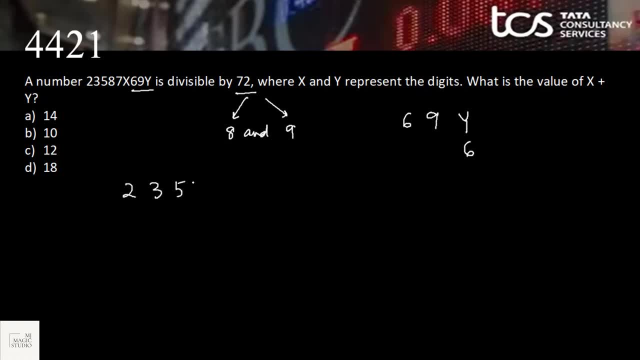 Value of y is 6.. 2,, 3,, 5,, 8,, 7,, x, 6,, 9,, 6.. Sum of digits: 9 gone, 8 to 10,, 1. And 8,, 9 gone. 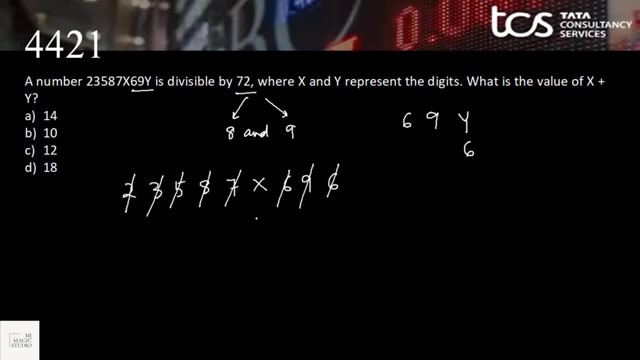 6, 6,, 12 is 3.. 3, 7 is 10,, that is 1.. So value of x should be equals to 8.. 7 plus 3 was giving us 10,, that was 1.. 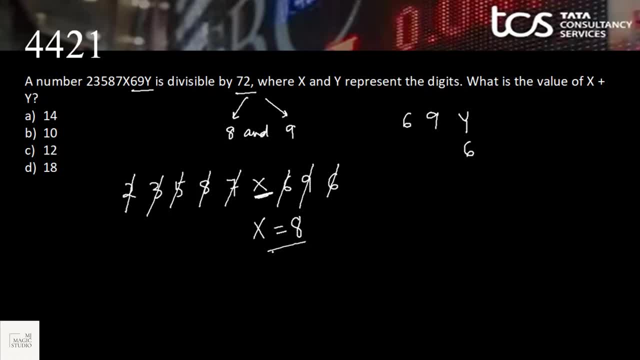 So 1 plus something should be equals to 9.. Value of x should be equals to 8.. So x is 8.. y is 6.. What is the value of x plus y? x plus y is 14.. 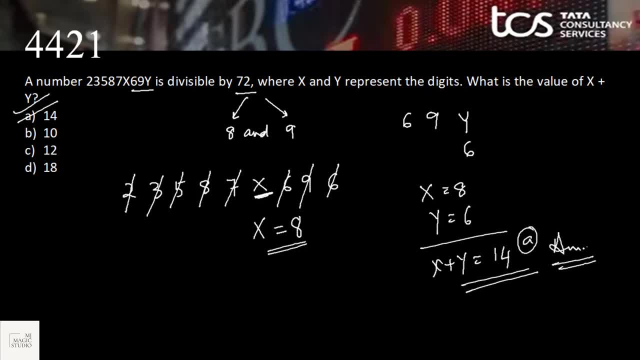 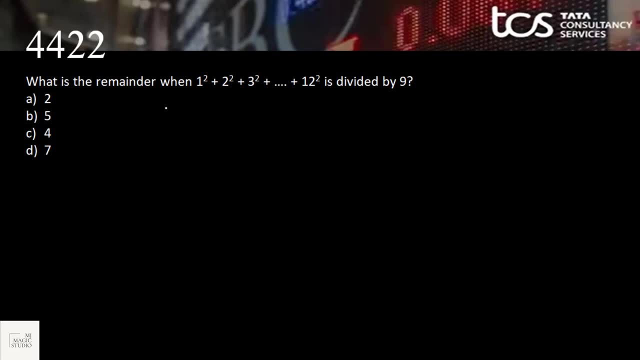 Option a is the pick. What is the remainder when this expression is divided by 9?? Whenever we are finding the sum of digits, the digital sum of digits is the remainder when it is divided by 9.. Suppose it is 13.. Digital sum is 1 plus 3.. 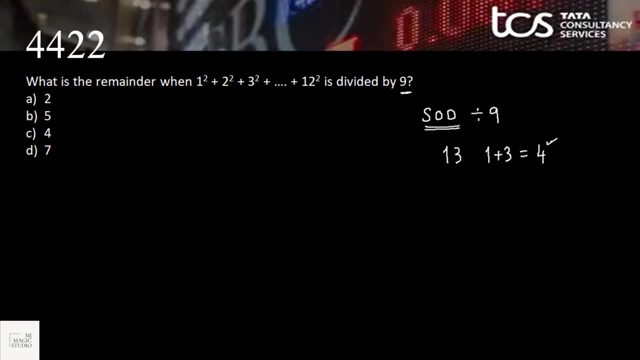 1 plus 3 is 4.. So when 13 is divided by 9, remainder is 4.. Suppose this is 3, 1, 8.. 3 plus 1 is 4 plus 8 is 12.. 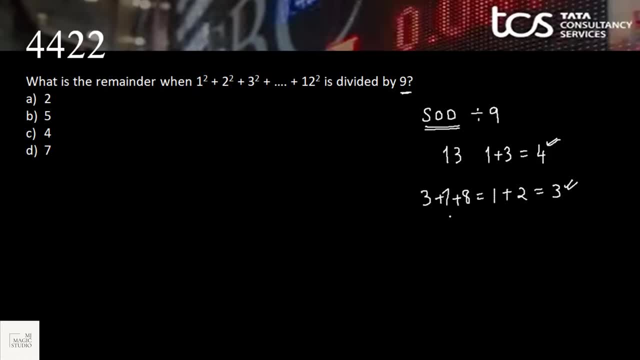 Now 1 plus 2 is 3.. So this is the remainder when 3, 1, 8 is divided by 9. That is known as digital sum. Now we also know that 1 is square, 2 is square till n is square is equals to n into n plus 1, into 2n plus 1 by 6.. 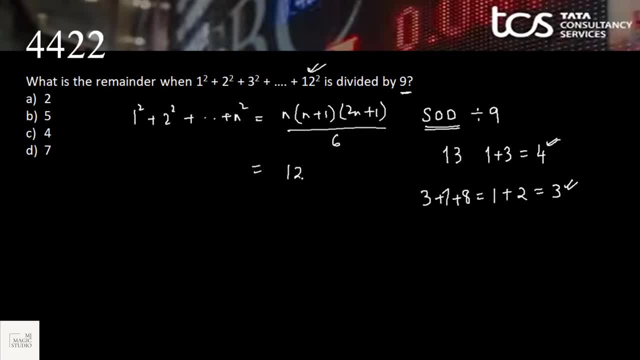 Here n is equals to 12.. So let us find the value first. 12 into 13, into 24, plus 1, 25 by 6. It is 13 into 50.. That is 650.. So sum of these number is 650.. 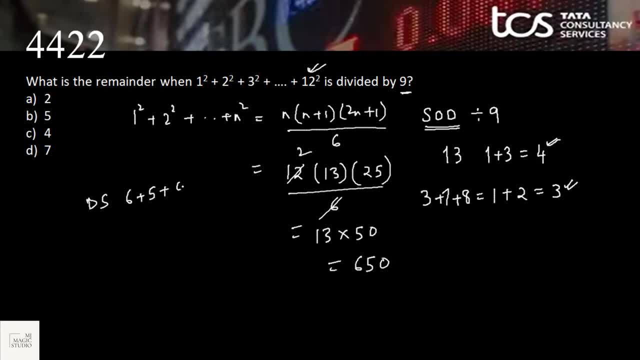 Digital sum of 650 is 6 plus 5 plus 0. That is 11.. That is 1 plus 1.. That is equals to 2.. That means when 650 is divided by 9, remainder is 2.. 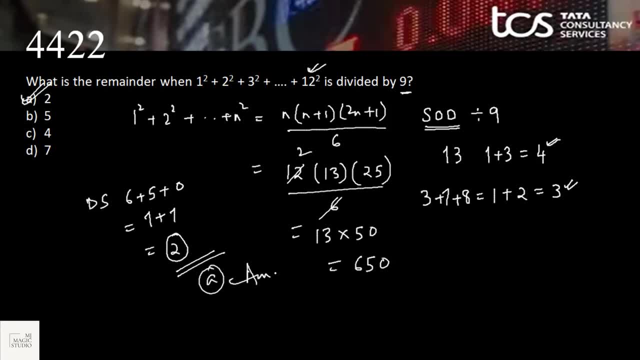 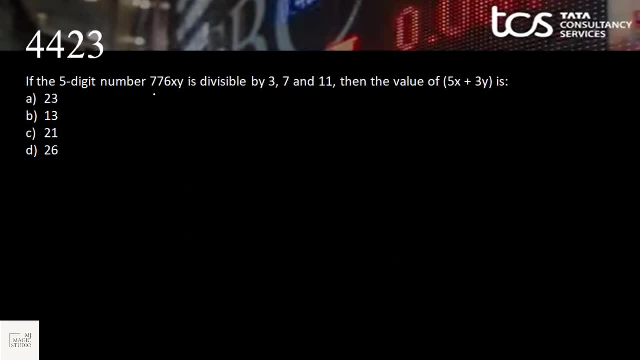 That is, in option A. We have a 5 digit number- 7,, 7,, 6,, x, y- And it is divisible by 3,, 7 and 11.. Then what is the value of 5x plus 3y? 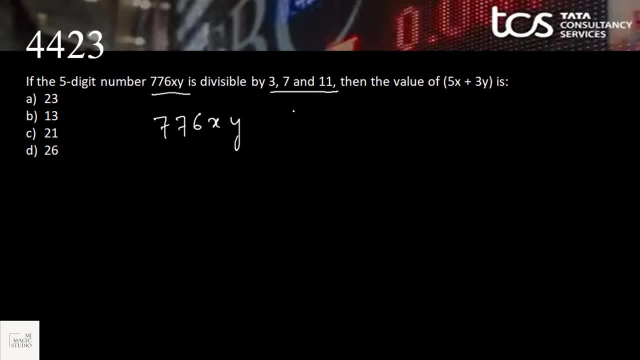 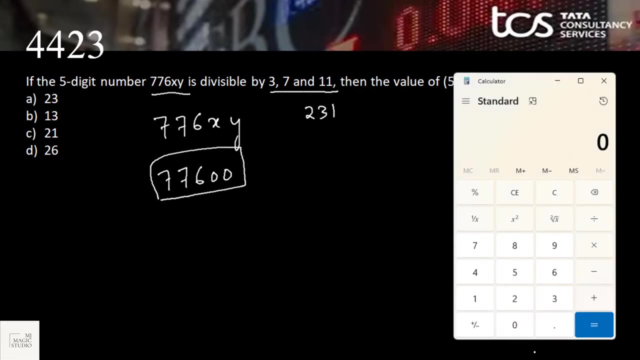 Now 3,, 7 and 11, all 3 are co-prime prime to each other. 3 into 7, 21 into 11 is 231.. That means this number is divisible by 231.. Let us take this number 7,, 7, 6, 0, 0 and find what number close to 7, 7, 6, 0, 0 is divisible by 231. 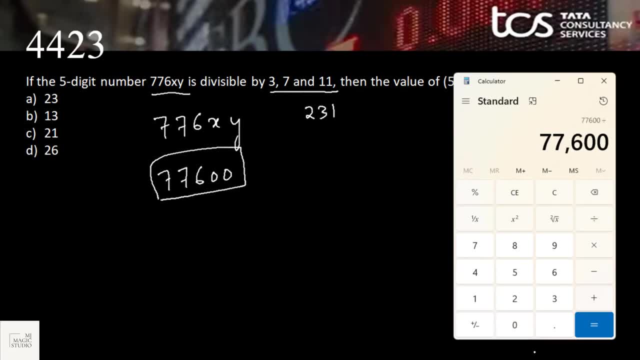 For which we have a calculator: 7, 7,, 6, 0, 0 divided by 231 gives 3.. 3, 35.9.. That means we are looking out for 3, 36 into 231.. 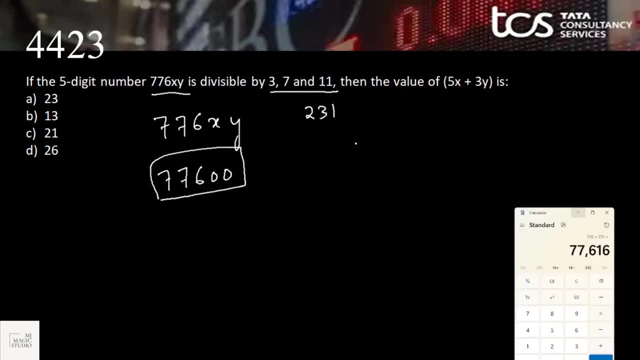 7,, 7,, 6,, 1, 6 is divisible by 231.. 7,, 7,, 6, 1, 6 is divisible by 231.. That means it is divisible by 3,, 7 and 11.. 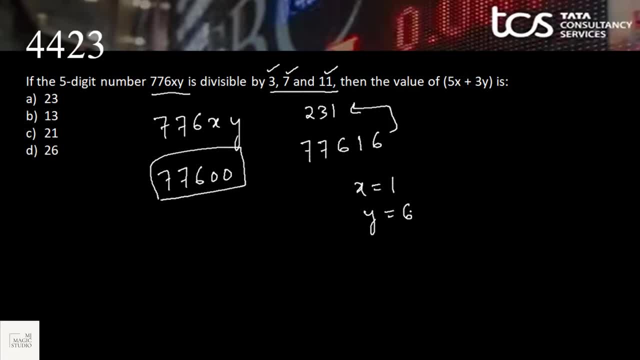 Value of x is 1 and value of y is 6.. 5x is 5 plus 3 into 6 is 18.. 18 plus 5 is 23.. Option A: Option A fits in On to the same kind of example again that we have done in the previous sum. 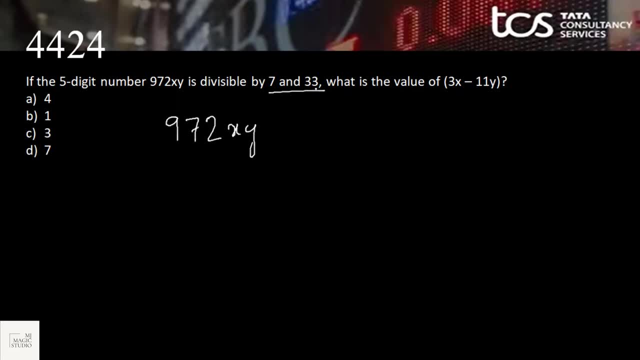 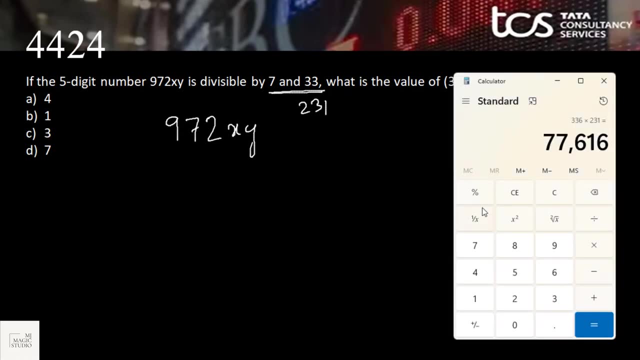 7, 9,. sorry, 9, 7, 2, x, y is divisible by 7 and 33.. 33 into 7, 231. again, Let me use my friend. So we have 9, 7, 2, 0, 0 divided by 231. 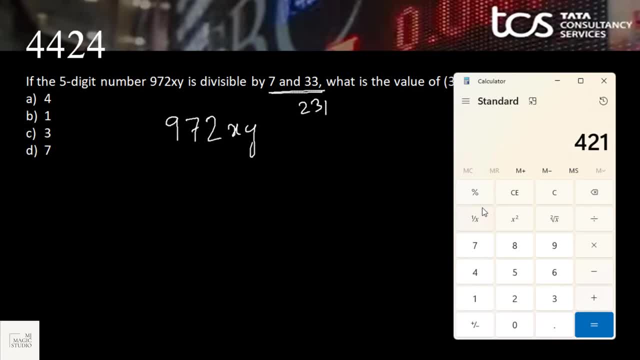 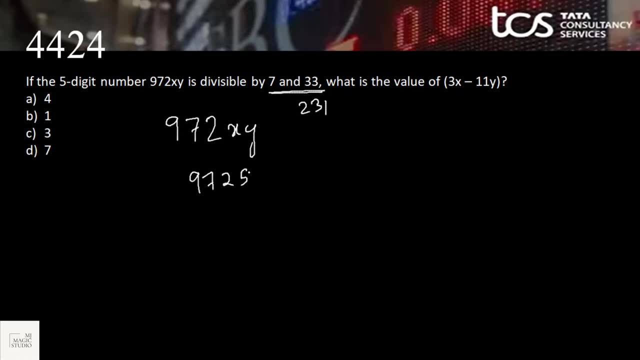 Is 4, 20.. So 4, 21.. 4, 21 into 231 is 9, 7, 2, 5, 1.. We have 9, 7, 2, 5, 1 is divisible by 231.. 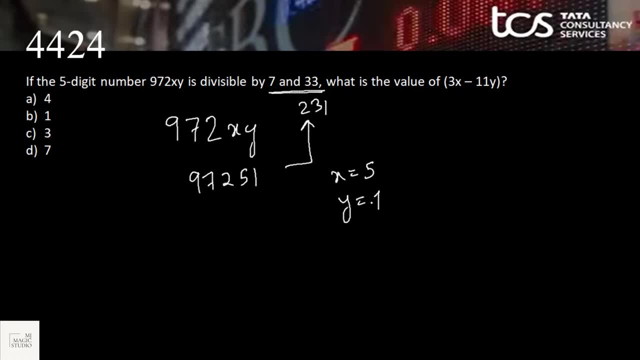 That means value of x is 5 and value of y is 1.. 15 minus 11 into 1 is 11, is 4.. Option A: Let's take up one more example. Okay, last simple question on divisibility rule on this section. 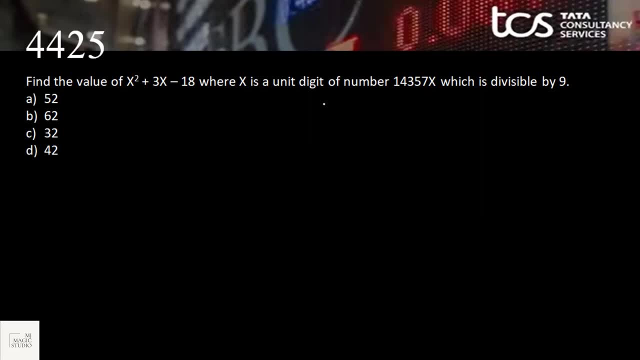 Let's see what we have. Find the value of a quadratic equation if x is a unit digit in the number 1,, 4,, 3,, 5,, 7, x which is divisible by 9.. We know that divisibility rule of 9, sum of digits should be divisible by 9.. 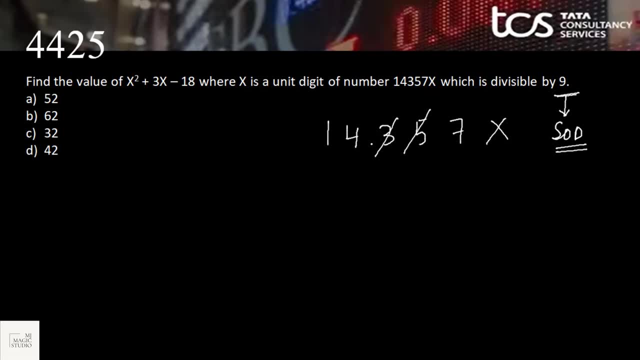 Let's find the digital sum 8 plus 7, 15.. 1 plus 5 is 6 plus 4, 10.. 10 is 1.. 1 plus 1 is 2.. So 2 plus x should be divisible by 9.. 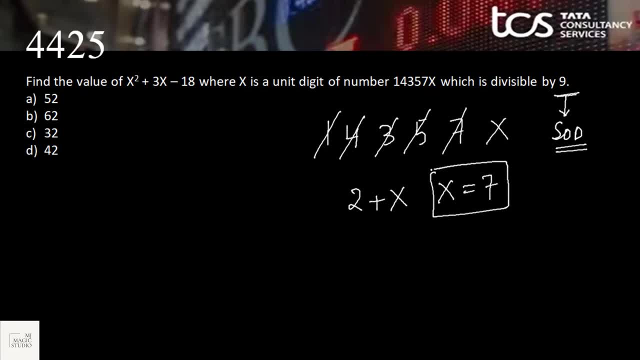 That means value of x is 7.. 7 square 49.. 7 into 3,, 21 minus 18.. 21 minus 18 is 3.. 49 plus 3 is 52.. Answer there in option A. 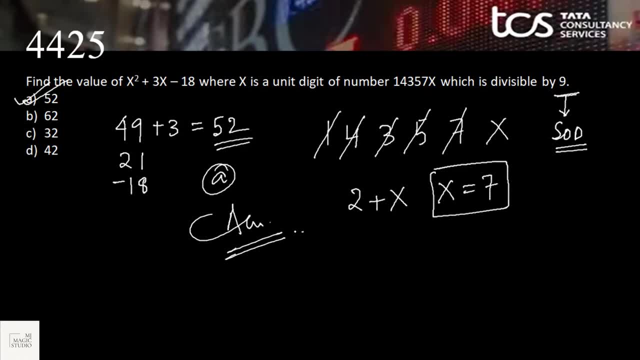 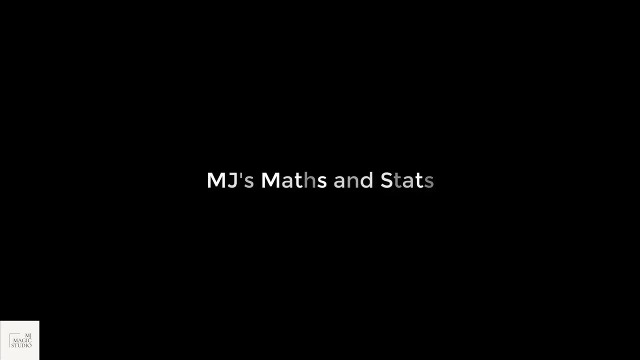 Do practice lot of divisibility rule, because TCS digital, TCS, NQT: Ask one question from divisibility rule and they will ask you questions of this format. So keep practicing questions like this. Thank you.